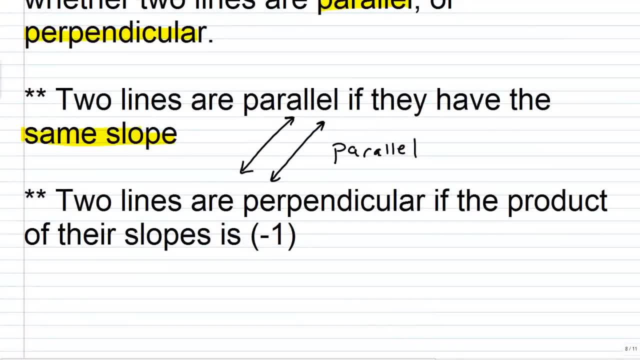 line. Okay, and then two lines are perpendicular if the product of their slopes is negative one. So perpendicular lines are going to intersect at a 90 degree angle. So if you graphed the lines, it would look something like this- And I know this isn't going to be perfect. 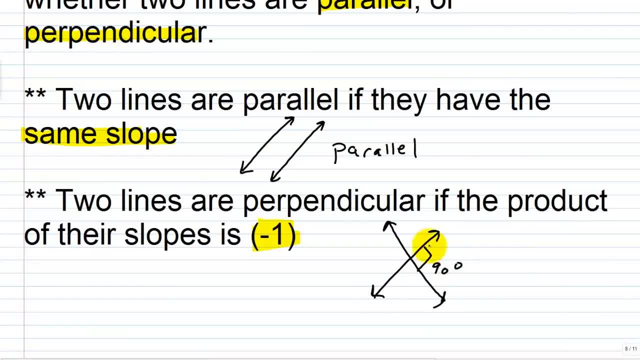 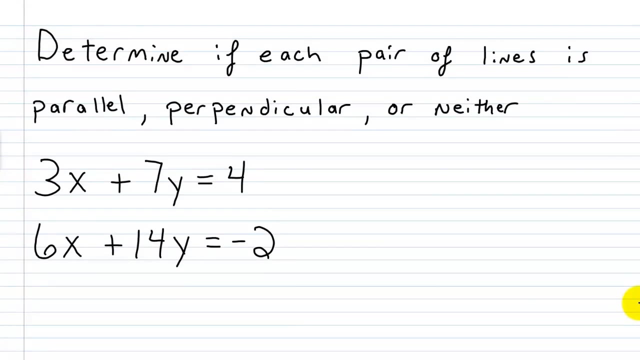 but it should. So again, two lines are perpendicular if the product of their slopes is negative one. So let's look at a little practice exercise here. I want to determine if each pair of lines is parallel, perpendicular or neither. So three angles. 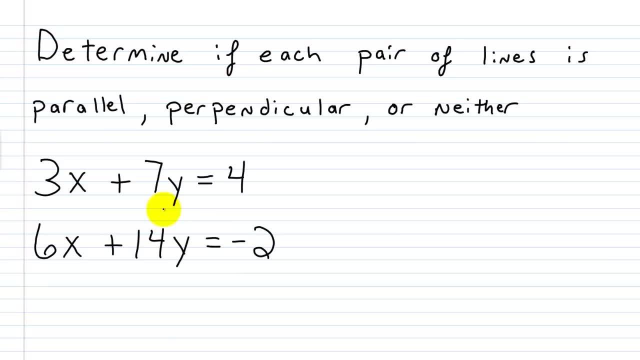 So 3x plus 7y equals 4 is our first equation, and 6x plus 14y equals negative 2 is our second equation. So all we're going to do is solve each for y and we're going to see what the 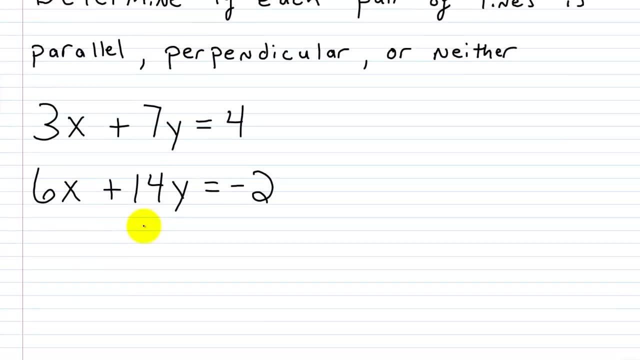 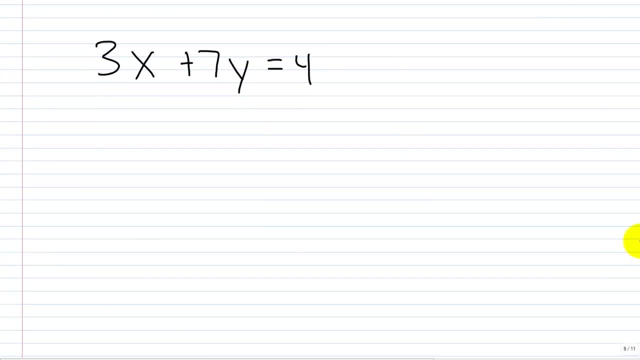 slope is. So we'll start with 3x plus 7y equals 4.. Let's solve this guy for y All right? so subtract 3x from both sides of the equation: We'll have 7y equals 4.. So we're going to. 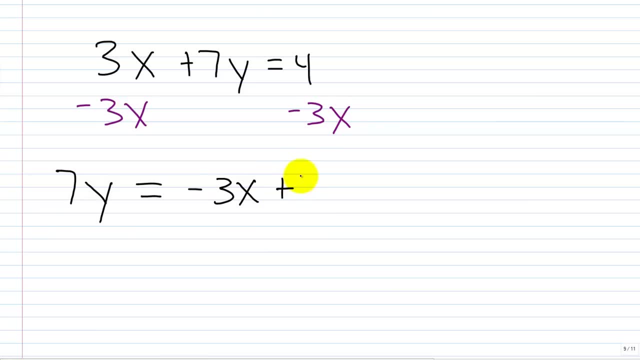 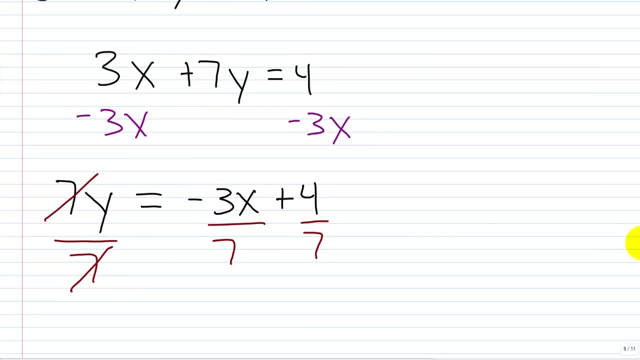 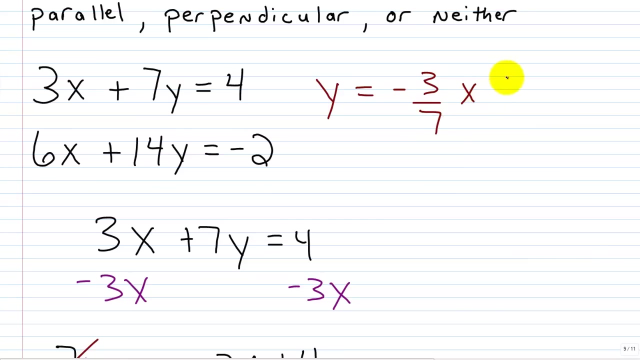 get negative 6y equals negative 3x plus 4.. And then I divide both sides of the equation by 7. And we end up with y equals negative 3 sevenths, x plus 4 sevenths. All right, now we have 6x plus 14y equals negative 4.. Now we're going to divide both sides of the equation. 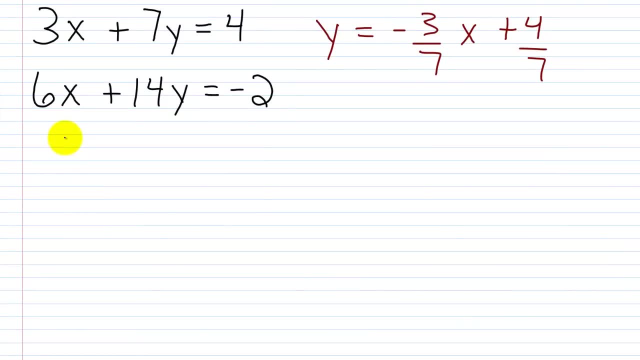 2.. And again, we want to solve this for y, So I'll rewrite this: 6x plus 14y equals negative 2.. We're going to subtract 6x from both sides of the equation And we're going to have 14y equals negative, 6x minus 2.. 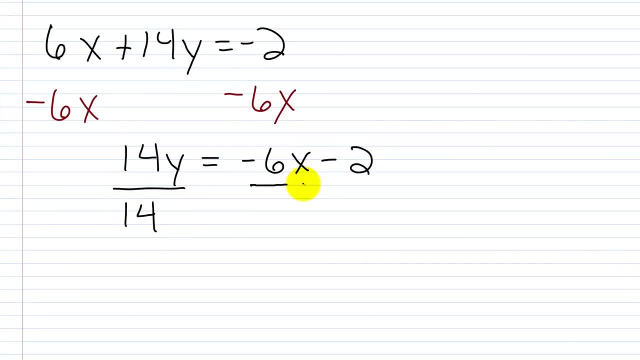 Okay, now we're going to divide each part by 14.. Okay, that's gone. We'll have y equals negative 6 over 14 times x minus 2 over 14.. Of course, I can reduce each fraction there, so let's do that. 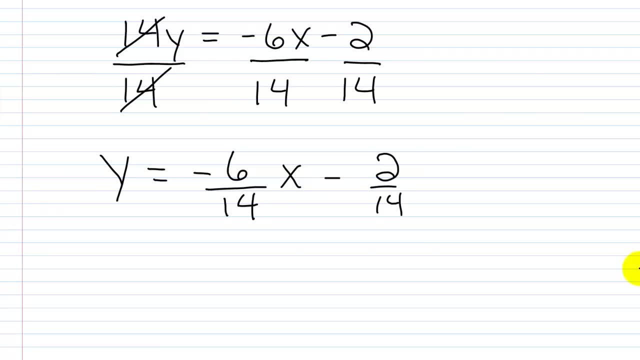 6 is 3 times 2, and 14 is 7 times 2.. So I can cancel a factor of 2 from both the numerator and denominator there. So I'll have y equals negative 3 over 7 times x minus. 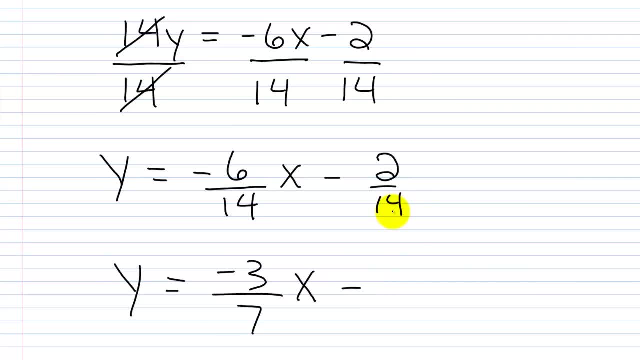 and then we'll have y equals negative 3 over 14.. So I'll have y equals negative 3 over 14.. And then 2 over 14. here I know 14 is 7 times 2, so this will be minus 1- 7th. 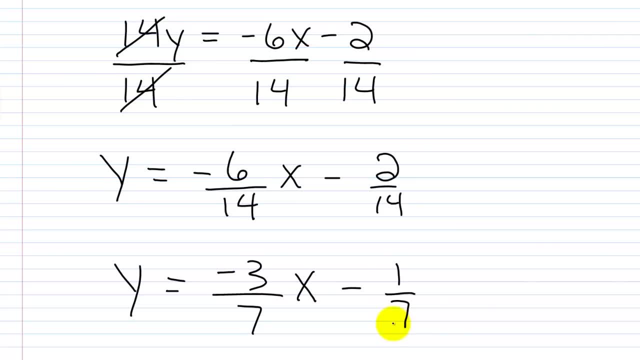 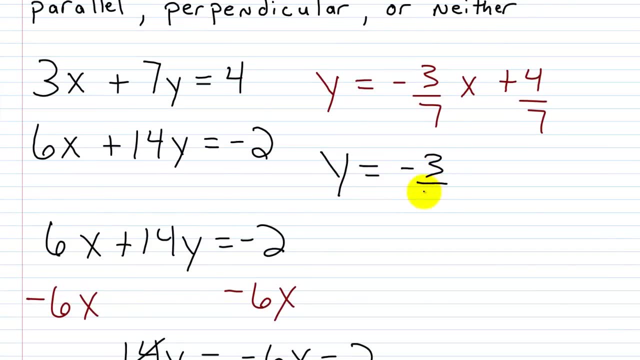 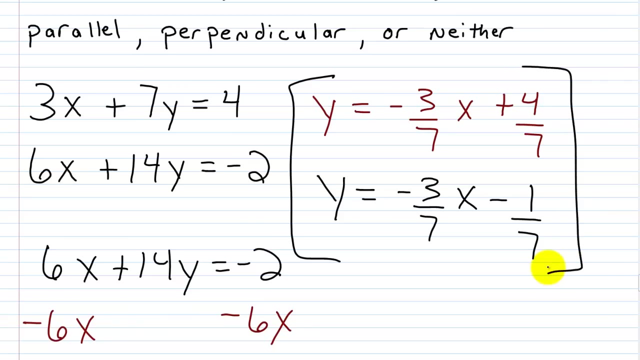 Okay, so y equals negative 3 7ths, x minus 1 7th. So you can see, now that we have our equations in slope-intercept form, it's pretty easy. The slopes are the same right And each of them are the same. 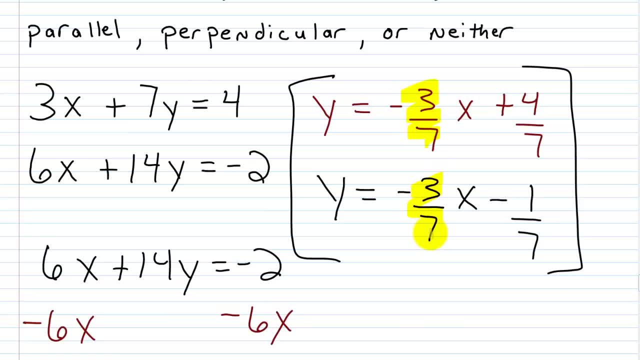 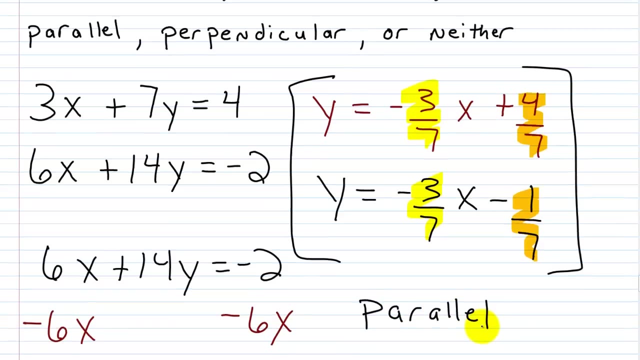 So in each case it's negative 3, 7ths And we have different y-intercepts so we know it's not the same line. So we'll say that these lines are parallel And again that's because the slopes are the same. 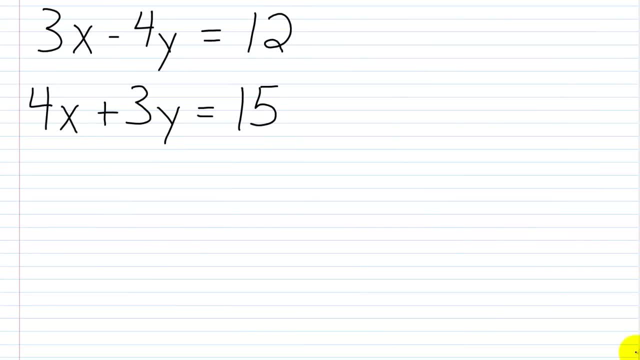 Okay for our final problem. we have 3x minus 4y equals 12, and we have 4x plus 3y equals 15.. So again, we're going to solve each for y to get it in slope-intercept form. 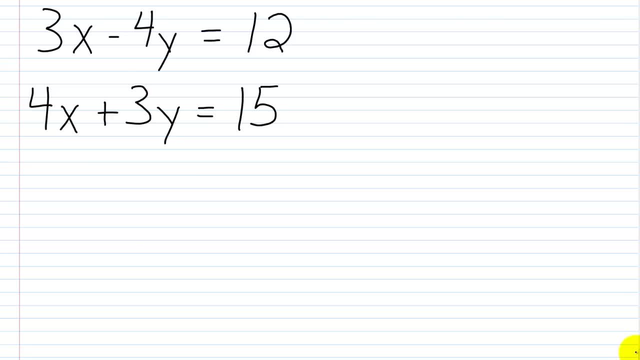 Then we're going to look at our slopes and see if we have parallel lines, perpendicular lines or neither. So let's see We have 3x minus 4y equals 12.. Start by subtracting 3x from both sides of the equation. 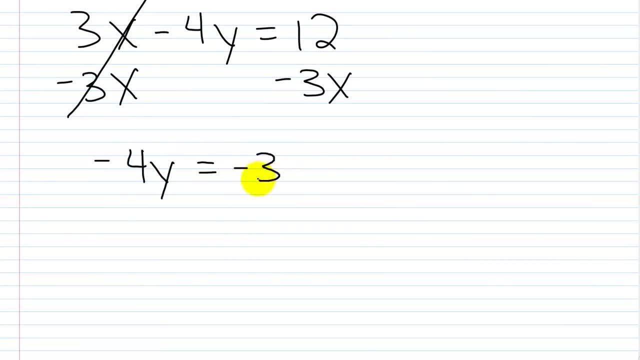 We have negative 4y equals negative 3x plus 12. And I divide each part here by negative 4.. Okay, that's gone. We have y equals negative 3 over negative 4 is 3 4ths right. 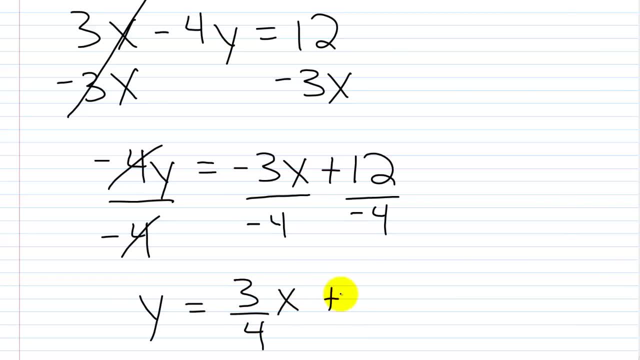 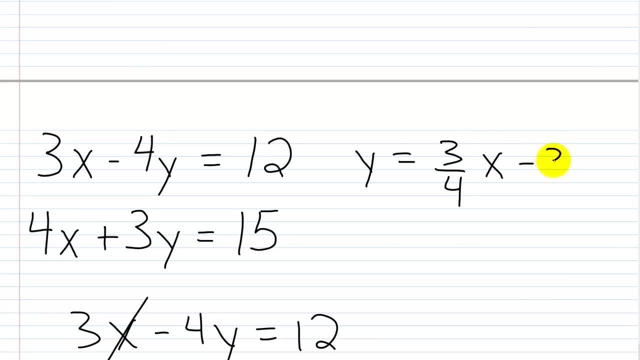 Negative over negative is positive. Then times x plus 12 over negative 4 is negative 3.. So I'm going to write this as minus 3.. So we have y equals 3 4ths x minus 3.. All right, let me erase and we'll get some room.